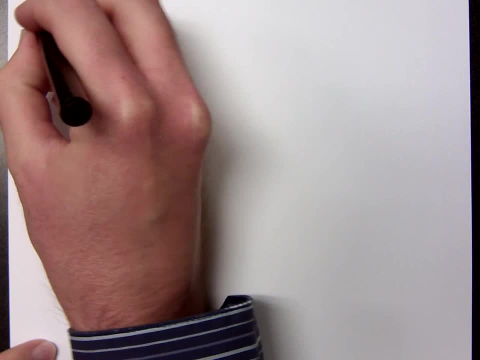 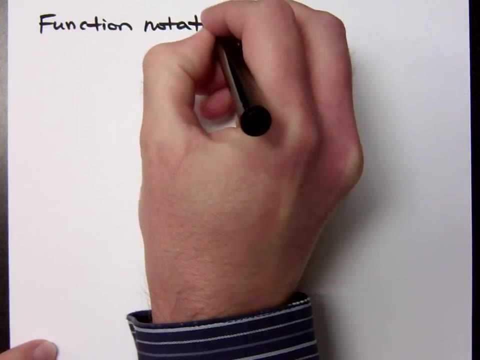 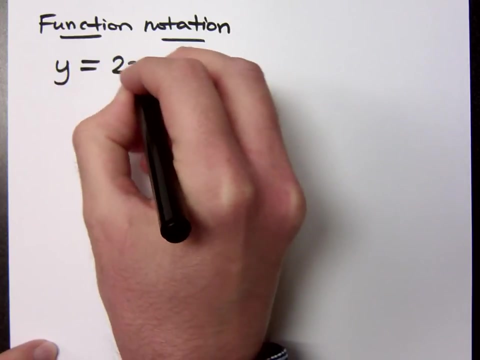 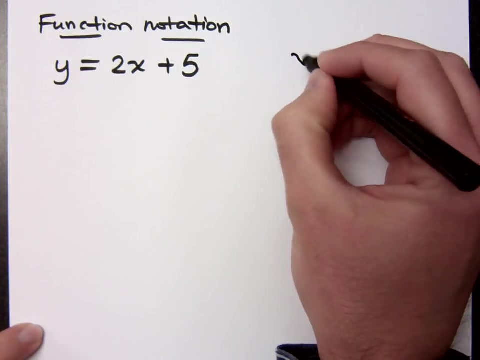 Now, right now, we want to talk about function notation And a lot of students get really confused on this and I don't really understand why. If I were to write this, if I said y equals 2x plus 5. If I did this and I said: you know what, let's make a t-table of values. 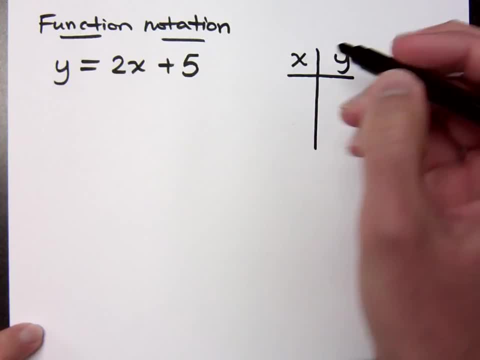 And I ask you guys to plug in, you know, an x value of 5.. Could you do it? If I asked you to make a t-table, could you do this? Yes, All right. what would you get for the answer? It should be 0, 5.. You get 15, right? If I plug in, x is 5, that means all you're. 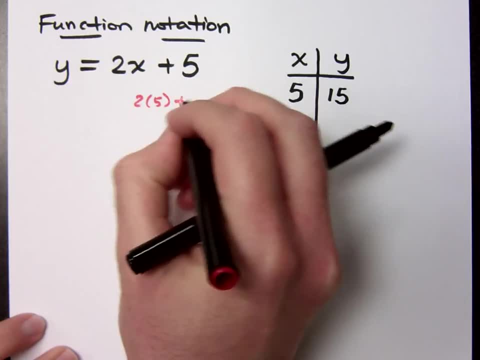 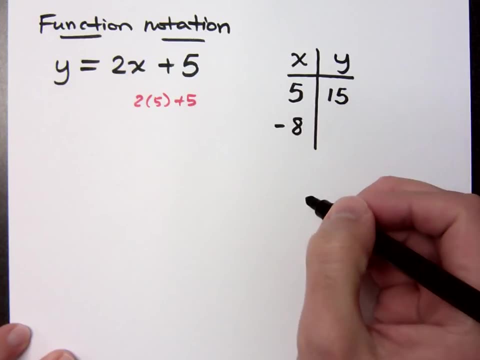 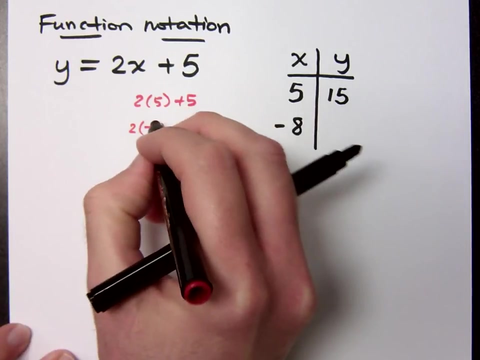 doing is x is 5.. All I'm doing here is 2 times 5 plus 5, right? If I ask you to plug in negative 8, that means 2 times negative 8 plus 5.. You know what? if you can't track this in your head, just 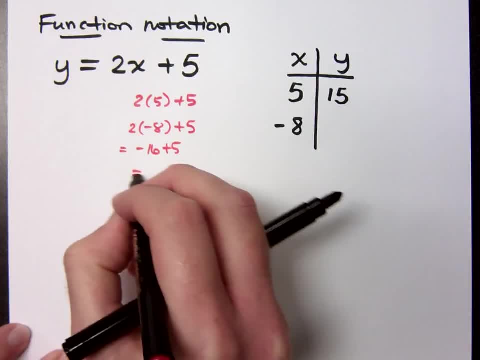 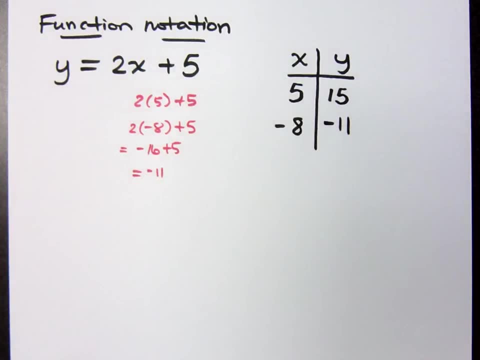 write it out. So that's negative 16 plus 5, which equals what Negative 11.. Now, if you guys aren't giving me any kind of any kind of mess about this, you agree with me about making a t-table like that? right, You just plug it in. If you can do that, then you can. 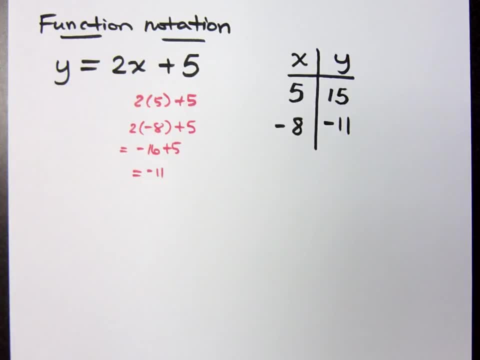 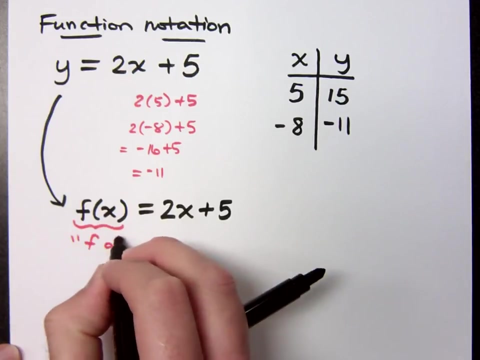 do function notation: See: instead of using y. what we'll see is this: This means the exact same thing: F of x equals 2x plus 5.. Please make sure that you understand that this guy right here you read this as f read. 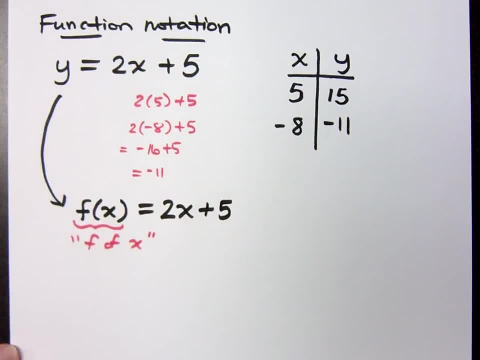 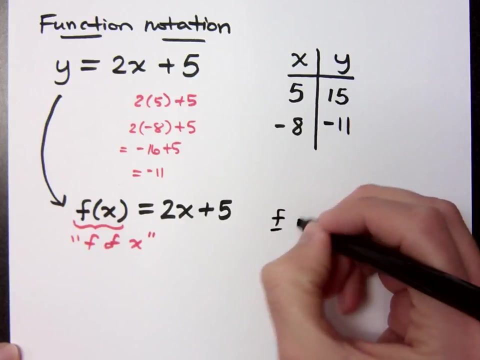 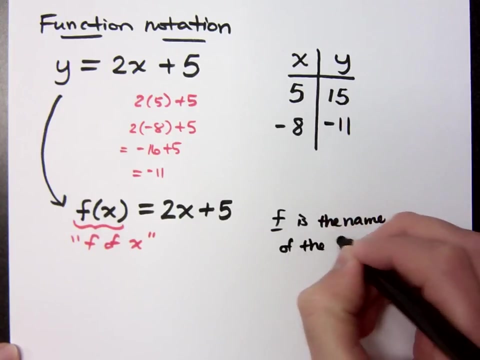 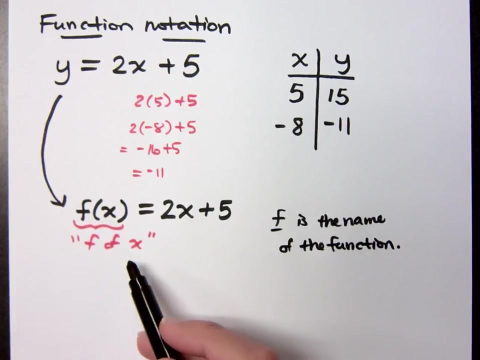 that as f of x. Okay, Don't say fx, Guys. you just sound unintelligent when you say that It's f of x. What this means is that f- f is the name of the function of x and it's based off the variable x. Now f is a common letter that we use for functions. 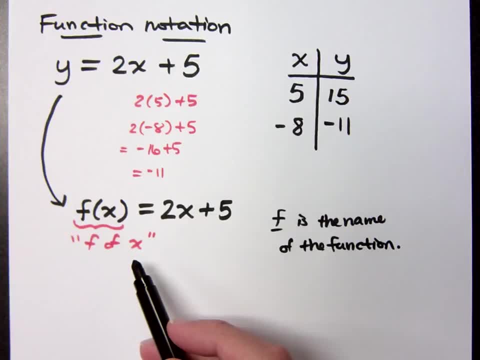 We may also use g and h or other letters that may, I guess, spark in our heads what's really going on Like. if we're talking about the cost function, a cost, we'll use maybe c capital letter, c of x. 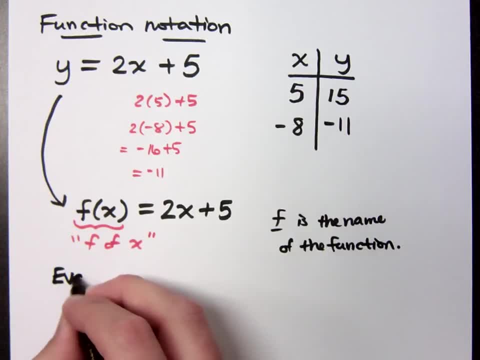 Okay, But I could take this guy and I could say: you know what I want you to evaluate the following: Evaluate f of 22.. Now, even though this says f of x equals 2x plus 5, this is just describing a rule and a relationship between x and the function itself, This function. 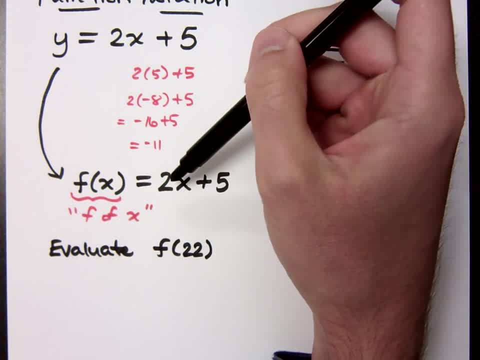 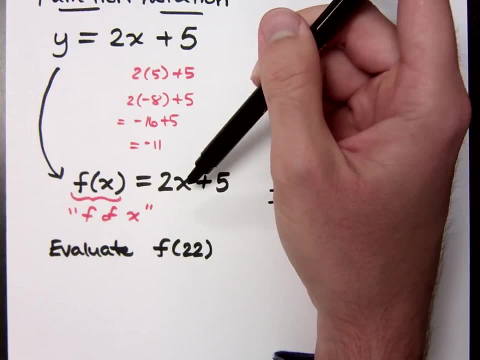 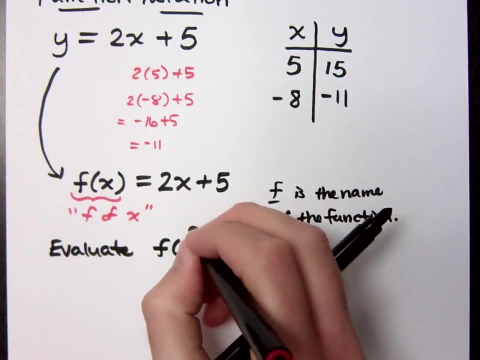 as you already knew from up here, tells me that if I want to find a value, if I've got it, if I know x, I plug it in here and I do the math right. So when I say this right here, f of 22, that means it's not x. This is my input value And this goes where my 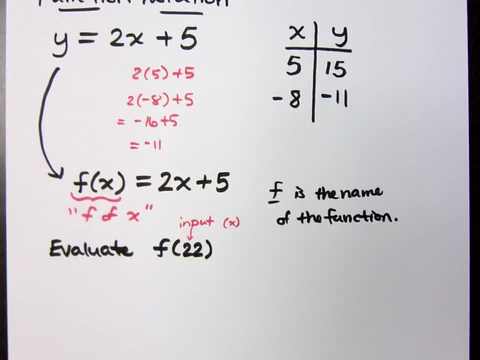 x was before. So this is what I want you to do. If you do it the exact same way that I'm showing you, then I won't ever be mad at you If I ask you to evaluate f of 22,. that means: 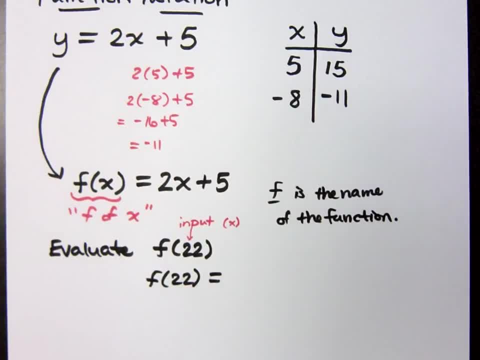 there's no longer x, And I'm taking out x and I'm putting in what 22.. I'm plugging in 22.. That's what that says. F of 22 says: replace the x with what's in there, which is 22.. So here's what I'm going to do. I'm going to do 2 parentheses plus. 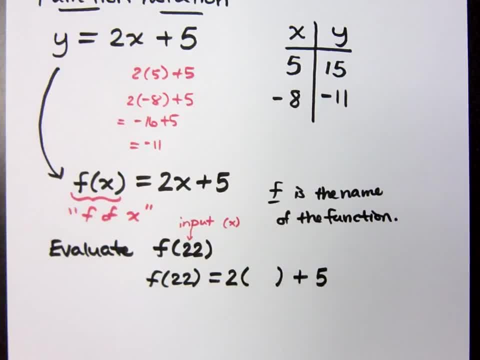 5. Anytime you do a substitution, you use parentheses. And what goes inside the parentheses? I'm concerned with plugging in 22, right, Mm-hmm? If you can't finish this, then you're in trouble. How does this get finished? What do you do? 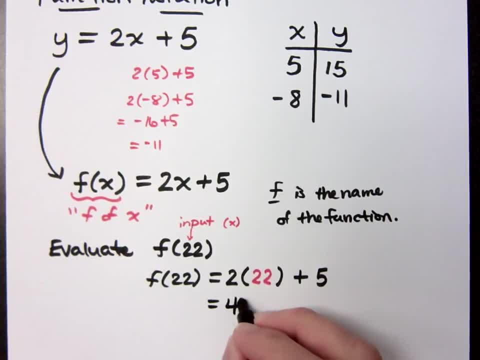 You multiply 22 times. You multiply this, You get 44 plus 5, and you end up with what? 29.. Now notice what I'm doing. I'm using my equal signs appropriately. I'm saying: f of 22 is. 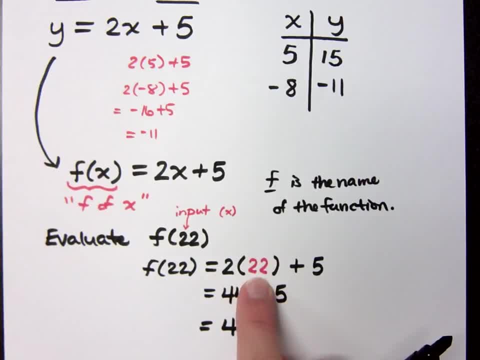 equal to this statement. where there's no x, I replaced it with the 22. Equals. that Equals this. Yeah, That's it Done. All right, If you want to, you don't need to say this, but if you want to, at the end you could. 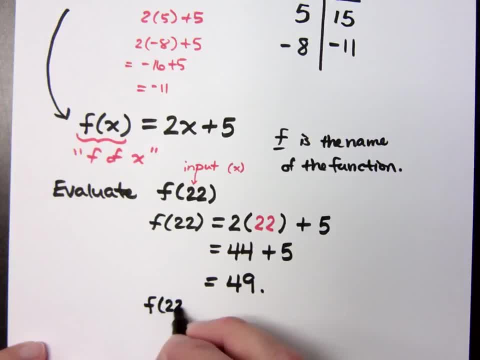 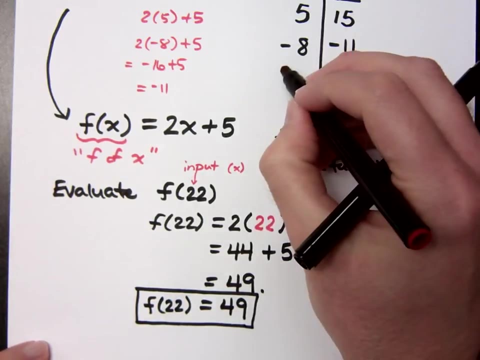 say this definitively: That f of 22 equals 49. You could say that You could deceive it like this: I don't really care, But think about what this means. That means that you, you plugged in 22 and you got what. 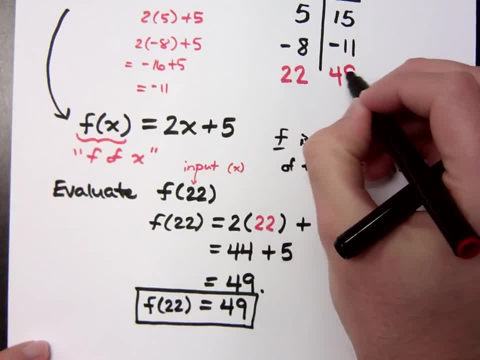 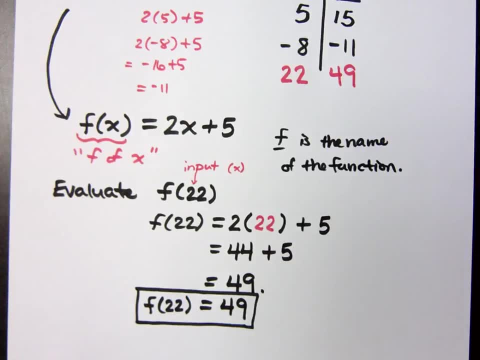 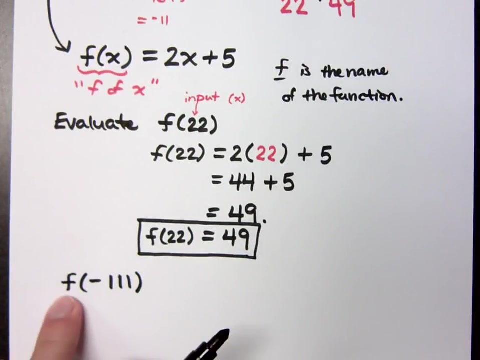 reek what we already knew how to do. We already knew how to do that right. So don't make this crazy, Don't make this scary If I say this: what is f of negative 111?? Notice that this f is referencing the most recent. 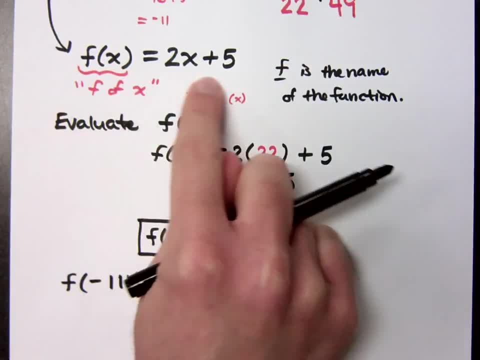 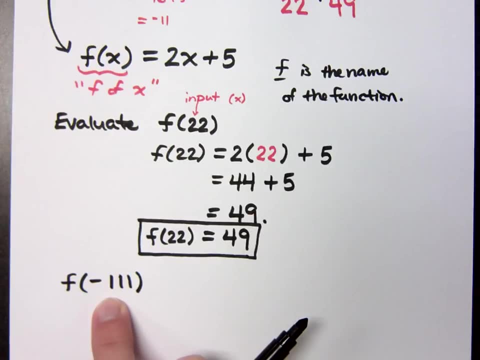 function named f. In this case, f of x equals 2x plus 5.. What does that negative 111 mean? That's what the x is being replaced by right. So here's what I want you to do: f of negative 11,, so 2, I'm putting in parentheses. 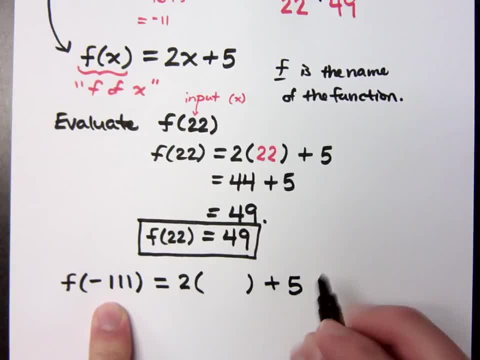 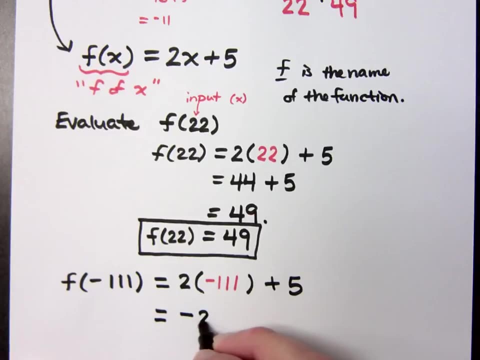 because I don't have x anymore, do I? What do I have in its place? I have negative 111. And it's just a matter of doing the math. So what do I have here? Negative 222 plus 5?. Negative 222 plus 5?. 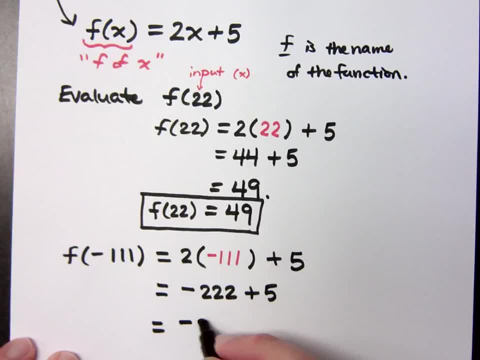 What is that Negative 217.. Are you with me on that? My question to you is: where is the x? Oh, there, it is Okay. The x is the negative 11,, 11, 11.. I mean 1, 1, 9.. 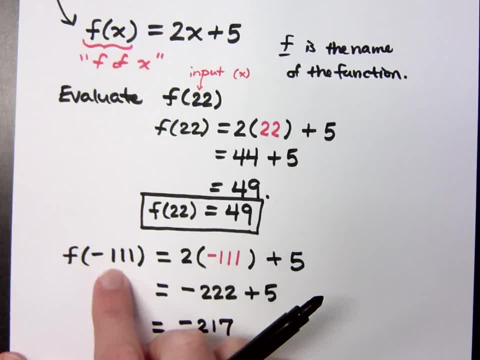 The x. well, this was the x value. The x was negative 111.. I replaced x with this guy right: Y is 217.. And the corresponding y value, or the corresponding function value, as we'll say, is negative 217.. 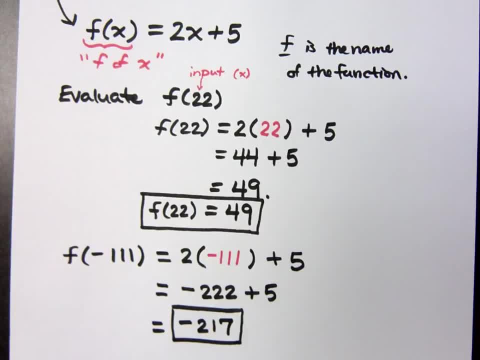 Notice what I did not do. I did not solve, I evaluated. Solving would mean at the end, x equals something, but that's not what it is. I plugged in a number and I got another number out. What do you think? 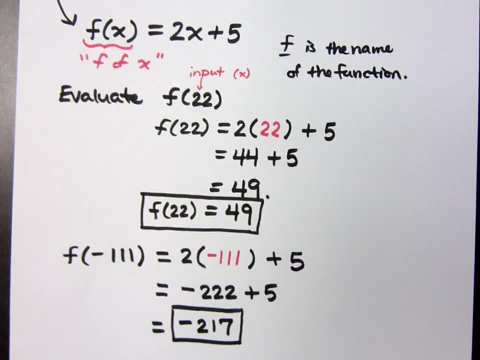 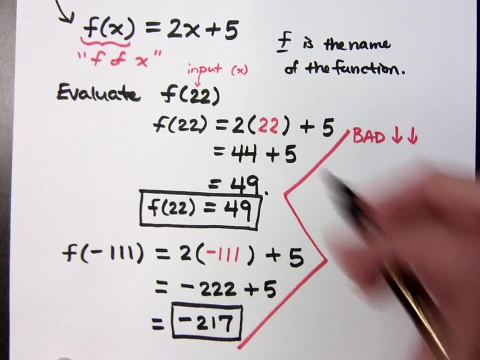 Now let me show you what bad people do. If you're doing this, then yes, you are a bad person. okay, This is what bad people do. okay, Bad people will say this: Oh, If f of 22 equals 2x plus 5,, this is what bad people do. 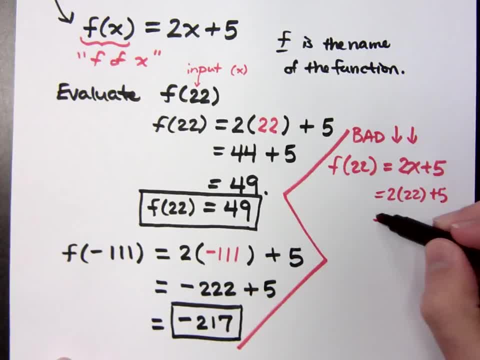 Drives me crazy. Now do you know why this drives me crazy? Because what equals 49?? Huh, I'm just curious. I don't see it. It doesn't finish. Well, you got 49.. That's the same answer that I got, right. 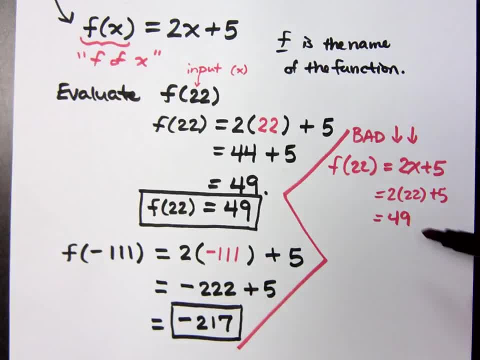 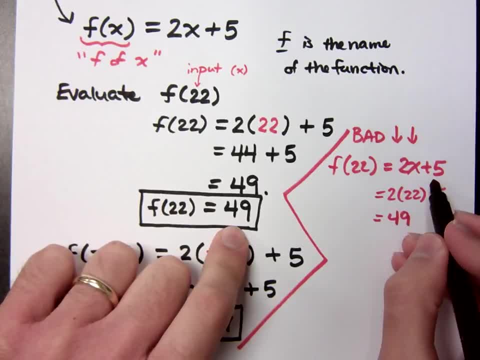 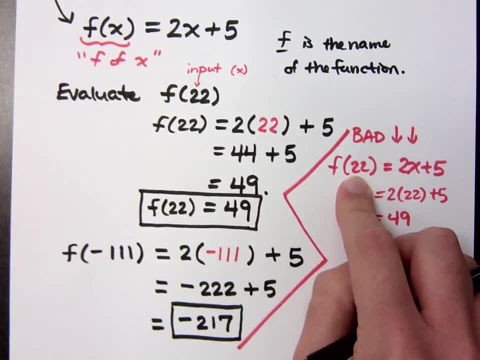 You didn't write down the f of x. This is wrong right here. Oh, because of the x, As soon as I have f of 22,. I no longer have x anymore, because x has been replaced with what? 22.. 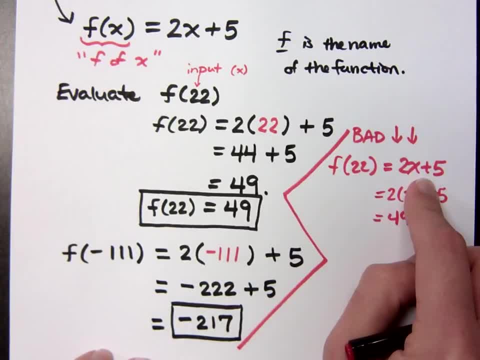 If you still write x, then you don't understand how to evaluate functions, and it makes me angry, So don't do that Now. what you could do is this: You could say this: You could say: f of x equals 2x plus 5.. 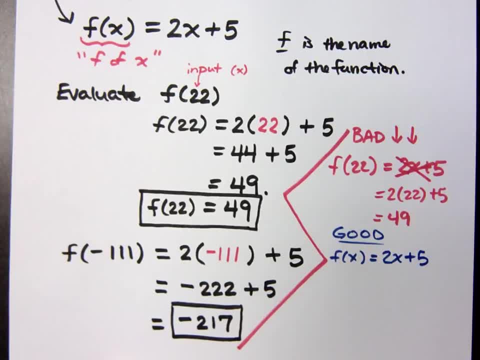 So if I ask you to evaluate, you write the original function and then underneath it you write: f of 22 equals 2 times 22 plus 5, blah, blah, blah, You get 49, right? Are you with me on that? 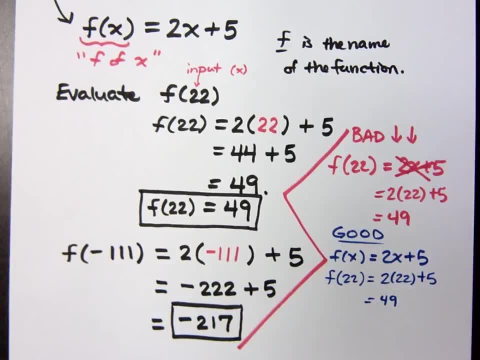 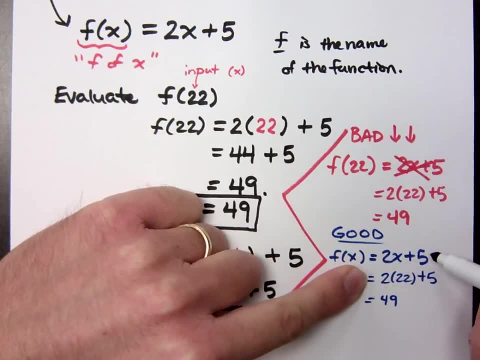 Mm-hmm, Notice what? Let me show you what would be wrong here. Okay, Okay, If they wrote this: does f of x equal 2x plus 5?? Yeah, it does right. Oh yes, Oh okay. 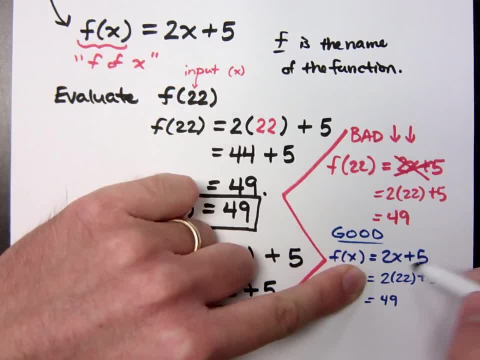 So this is not a bad statement, But does 2x plus 5 equal 2 times 22 plus 5?? No, This is a variable expression. That's my. I guess that's my template, so to speak, Here. if you don't have f of 22,, then you're wrong. 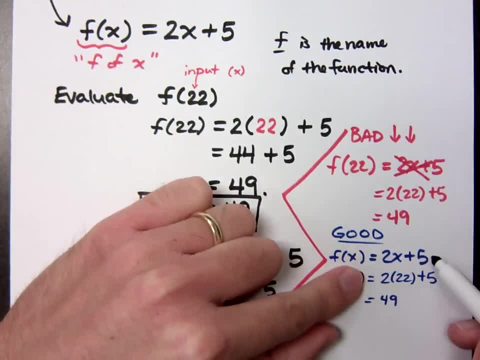 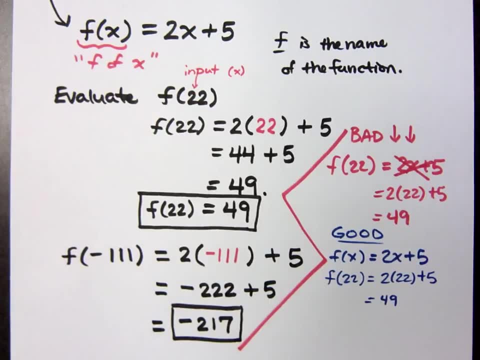 And you're basically telling me this. You're basically saying that 2x plus 5 is equal to 49.. Does 2x plus 5 equal 49?? No, 2x plus 5 is a variable expression, So this value is not set. 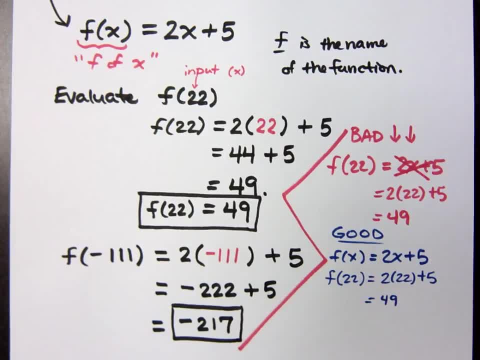 It can change. So when I evaluate, I'm plugging in different numbers. Are you with me on that? Yes, Let me show you something else that's bad. People will do something like this. blah, blah, blah, blah blah. 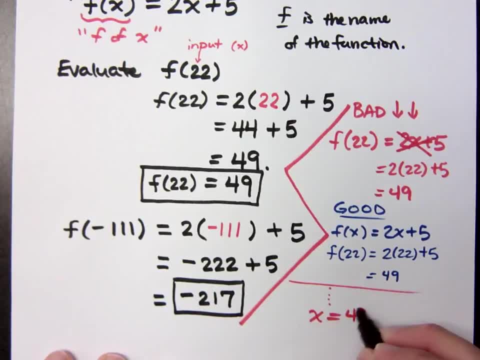 Ah, Okay, X equals 49. Okay, Okay, Okay. No, it doesn't. You're letting x become 22, and you're evaluating right. Don't do this. Let me show you something else that people do. 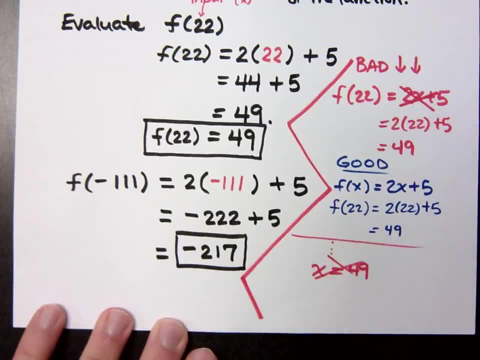 Again, if you find yourself doing this, you're wrong And I'll see you in the same class next semester. Oh, so it's 22,, so I need to do this. Show it back. You got to make me upset. 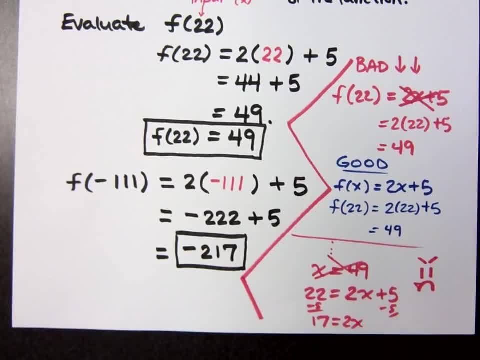 This is wrong. I don't want to say this is stupid, It's just really wrong. Okay, You're not solving You. don't do that. You do it the way I showed you. Are you with me? Yes, If you don't like this, go back and watch this video so you can hear me rant again.